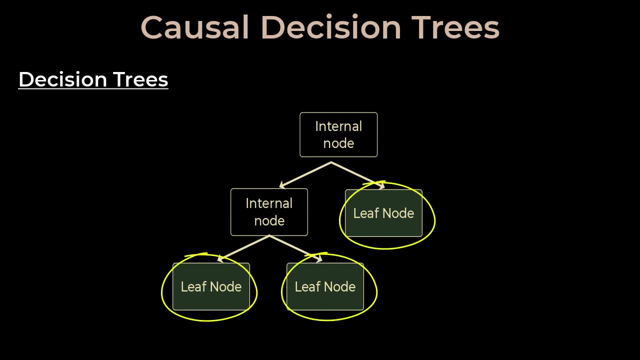 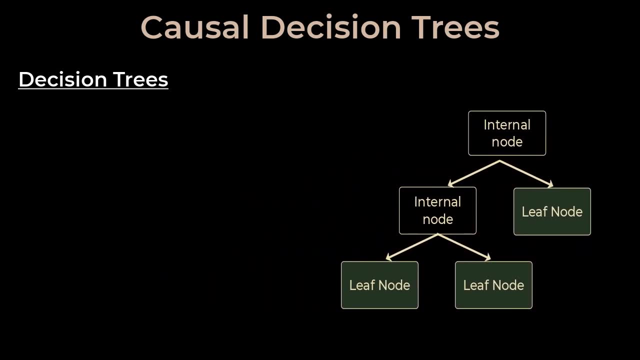 that have children and external nodes or leaf nodes that have no children. Let's illustrate how decision trees work. Let's illustrate this with a medical example. The flu is a problem for the world and I developed an elixir that I think should cure the flu, But before releasing it to the world, I want to test. 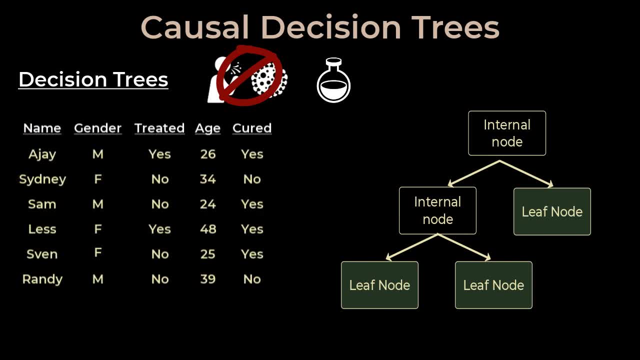 if this elixir works, And here's data for six people who came to me with the flu. For each person, we're tracking their gender, whether they were treated with the elixir, their age, which is a continuous variable, and finally, if they were cured. 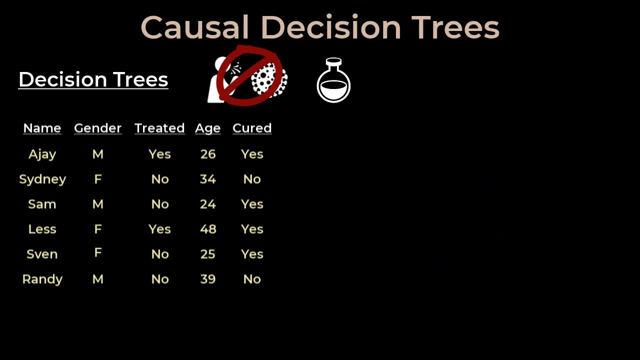 Let's say we have this decision tree to determine if a given patient will be cured. Let's take the first sample, Ajay, and see how this works. So Ajay is going to be passed to the root of the node. at the top, His age is checked to determine if it's above 30. It's not, So we 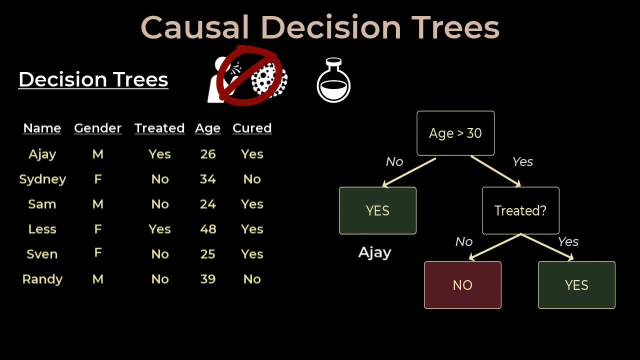 go to the left leaf node and this indicates that Ajay will be cured. It's a prediction. Now let's take our second patient, Sydney. She's passed into the root node at the top. Ajay is checked to see if it's above 30. It is above 30, so we go to the right child. 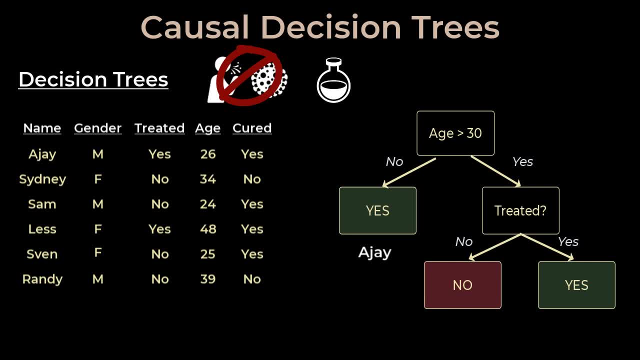 And this is another internal node where we check if the person is treated with the elixir. They were not And we predict that this person will not be cured. So let's take a look at the second patient, Sydney. She's passed into the root node at the top And we 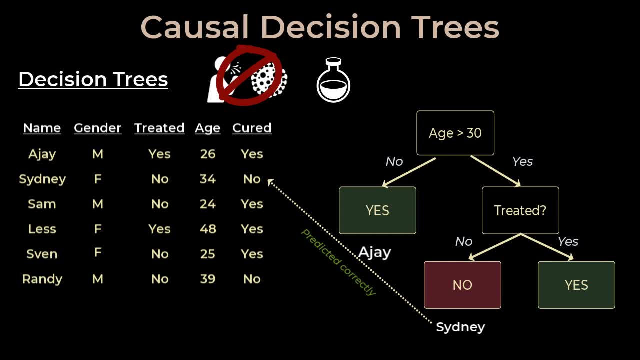 similar way, we can make decisions about whether a person will be cured or not by passing them down this tree and seeing which leaf they end up in. So this is pretty cool, But how exactly did we build this tree? The leaf nodes should be one of two outcomes: Yes, this person will be cured, Or 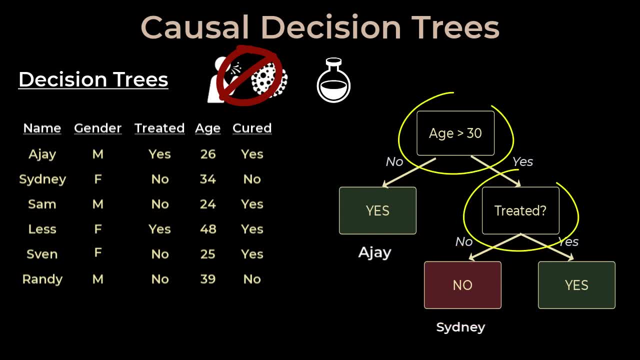 no, this person won't be cured. The internal nodes can be based on one of three variables: gender, whether the person was treated with the elixir, or the age, And the goal here is to choose internal nodes that can best split the yeses from the noes. 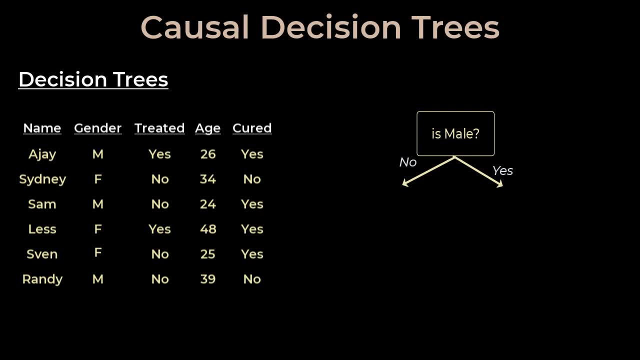 Let's start with gender as a potential internal split node. If we pass all the patients into this node, we'll end up with two yeses and one no on the left child, And then we'll end up with two yeses and one no on the right child, And then we'll end up with two yeses and one no on the left child. 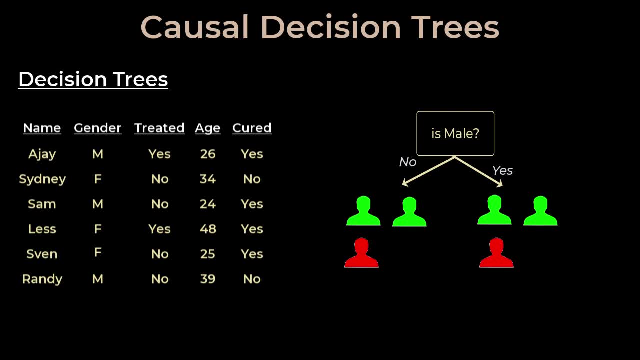 And then we'll end up with two yeses and one no on the right child. Instead, what if we started with whether the person received the treatment or not as the root? If we pass in all the patients to this node, we'll end up with four treated individuals on the left, two of whom were cured. 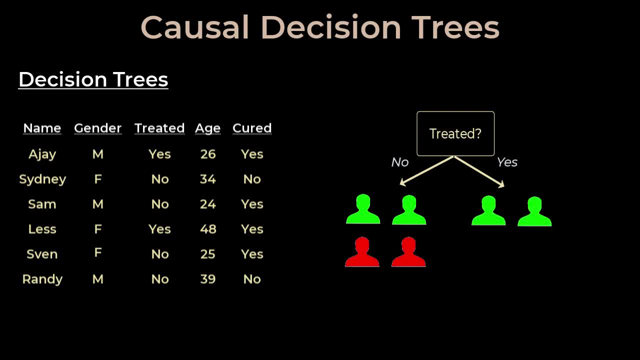 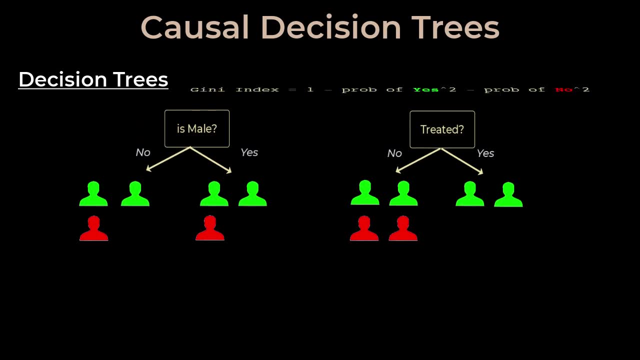 and two were not, And we'll end up with two cured individuals on the right. So which split is better? And we can quantify this with the Gini index. So Gini index is going to be one minus the probability of yes, square minus the probability. 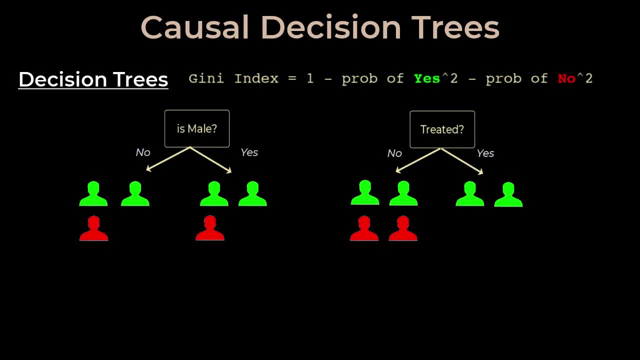 of no square Gini index is a measure of impurity. Lower the value, better is the split subject to overfitting. The Gini index of a split is the weighted average of the Gini index of each child node where the weight is going to be the total. 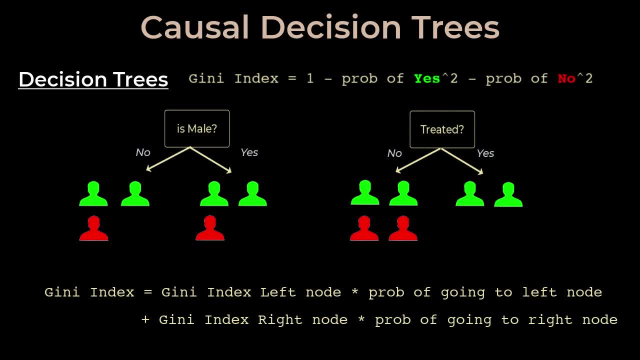 proportion of samples that are in that child node. This might be a little weird to understand at first, but let's walk through this by calculating the Gini index for the gender split and then the treatment split Before we move on. if you do like what you're hearing right now and 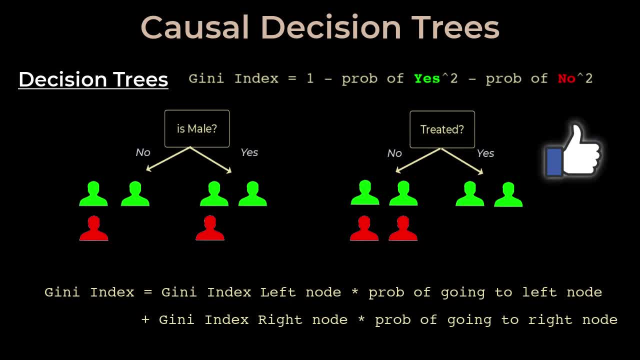 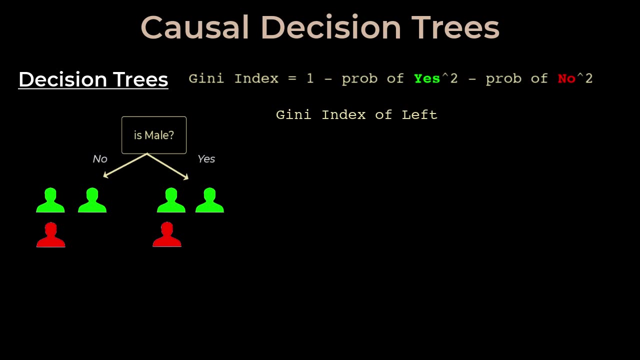 you want to know more. please do give this video a like and also subscribe and share it with people that you know, because it would really mean a lot to me. So let's consider the gender split. The Gini index of the left node is one minus the probability of yes, square minus the probability. 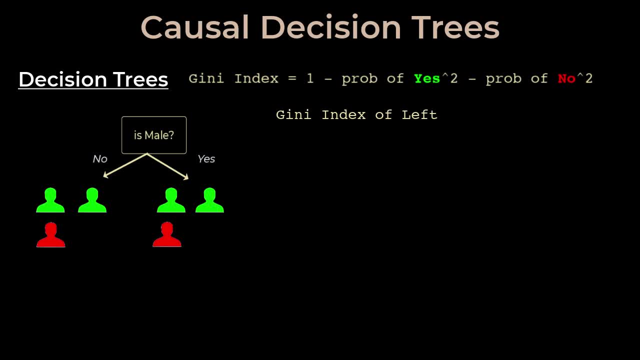 of no squared. So in the left node we had two yeses and one no. So the probability of yes is going to be two on three, where three is the total number of samples in the left node, And similarly the probability of no is going to be one on three, since there were 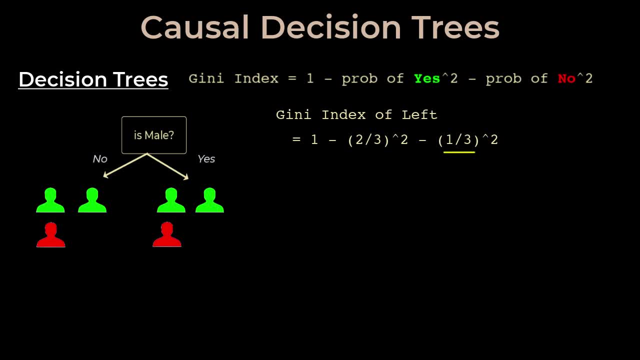 three people. And so we get the Gini index of the left node as 0.44.. And since the situation is exactly the same for the right node, we also get the Gini index as 0.44 for the right node. Now to compute the. 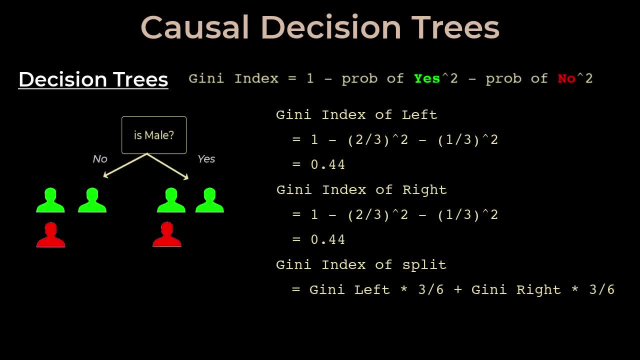 total Gini index. we take the weighted average of the Gini indices of the left node and we get the weight difference between the no less than or equal to zero, which we convert to zero at four times. So we're going to make a variable called 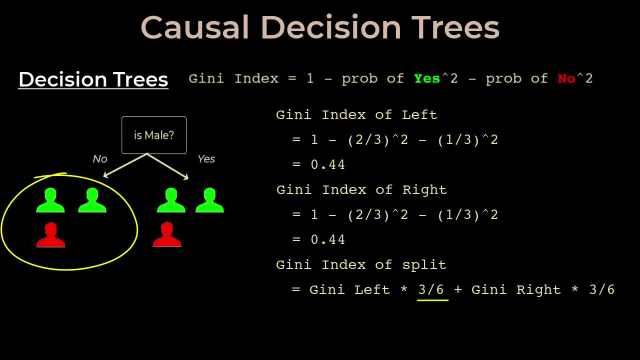 Zero plus four. zero plus four. Zero plus four is the difference between the weight, difference between the weight of the left node and theSpace elections. So step one for me is just going to control the Gini index. We're going to put it in the right node and we're going to change theρό similarly. 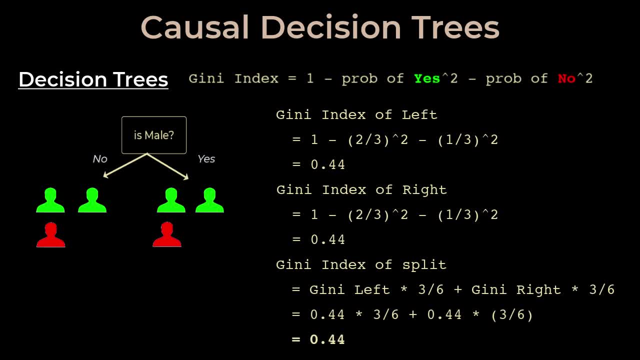 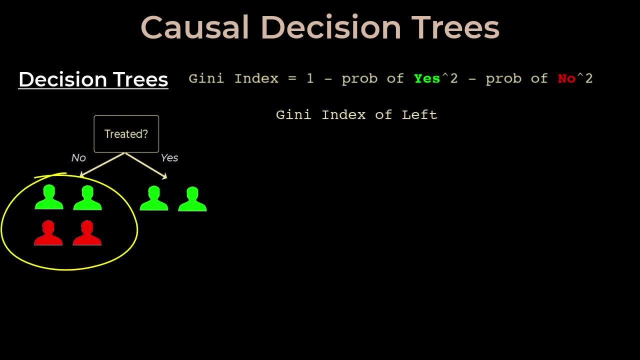 here to say: red equals 16. And then theZero equals 16.. And theZero equals 16.. So we will. Now let's compute the Gini index for the treatment split. So on the left node we saw that there were four treated individuals that went to the 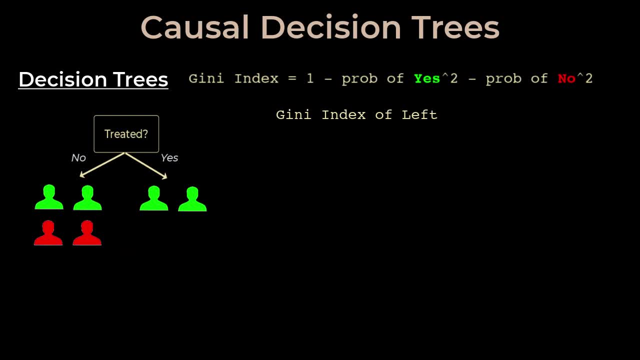 left, two of whom were cured and two were not. So the probability of yes in the left node is two on four and the probability of no in the left node was also two on four, And substituting these values, we get the Gini index of the left node as 0.5. 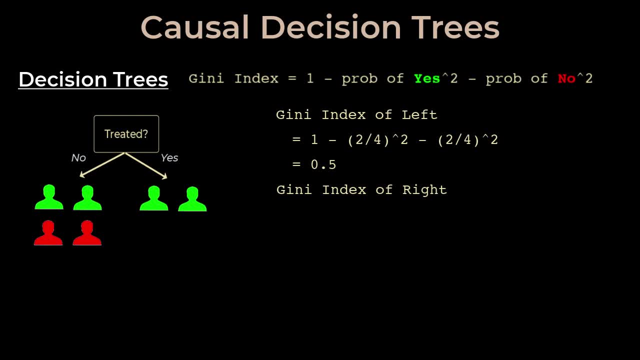 Now let's do the Gini index of the right node. Now for the right node. there were two individuals that went there who were eventually cured. So the probability of yes is going to be two on two and the probability of no is well. 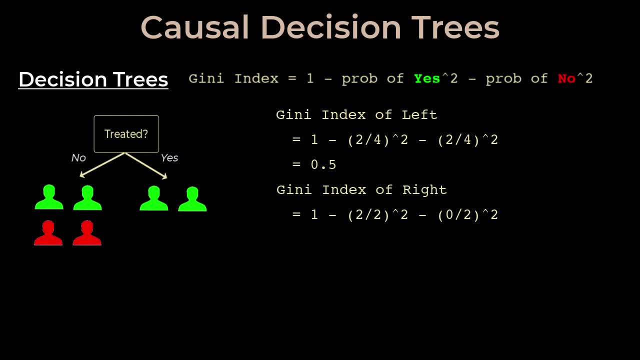 zero on two And substituting these values, we get the Gini index of the right node as zero. Okay Now, since we had four individuals who went to the left node out of six, that is going to be the weight of the left node. 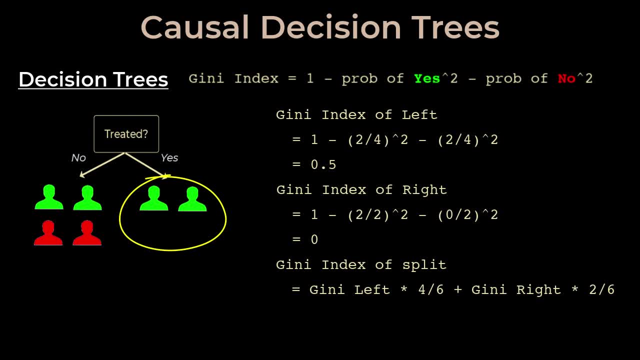 And two people out of six went to the right node. so two on six is going to be the weight for the right node And substituting these values we get the total Gini index for the treatment node as 0.33.. From these calculations we see that the Gini index of the left node is zero. 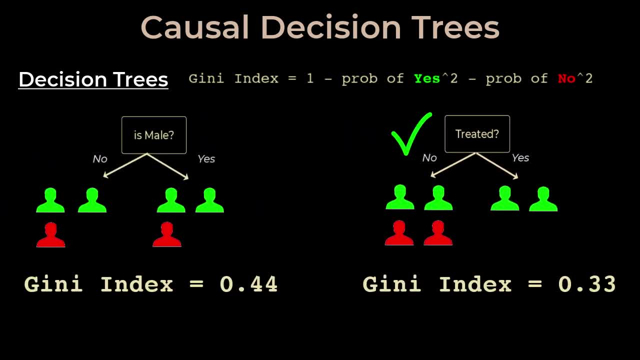 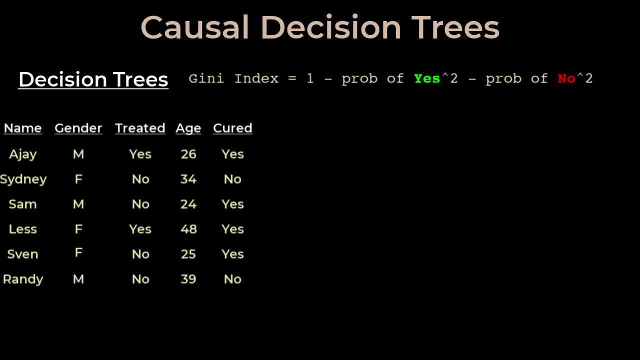 So we see the treatment split is the better split since it has a lower Gini index. Let's compare this now to the age split. The split for age isn't apparent, but we can get splits with a few simple steps. So we take the age of all individuals, sort those ages in ascending order, determine the 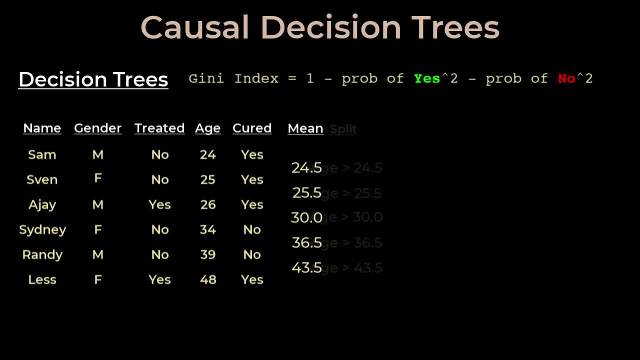 average age of subsequent entries and use each of these as potential thresholds to determine the age possible. We get the gini index of the left node as zero. So this is similar to using a split for the treatment determine Gini indices. So let's take the first case: age is greater than 24.5.. 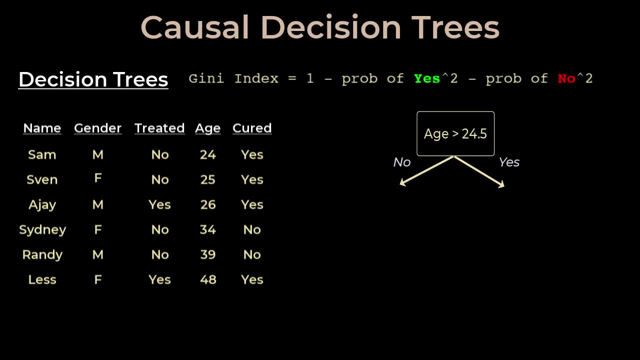 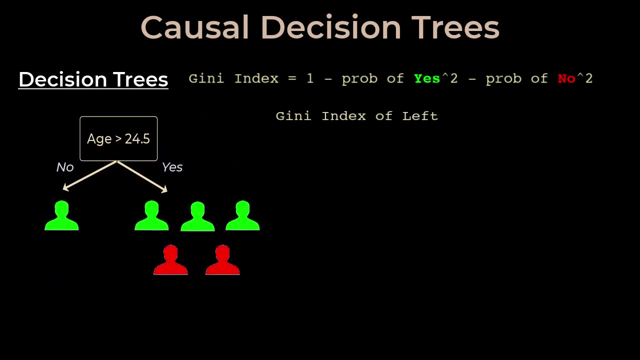 If we pass all the patients into this node we'll end up with one yes on the left child and three yeses and two noes on the right child. We now compute the Gini index of the split. So on the left child we had one. 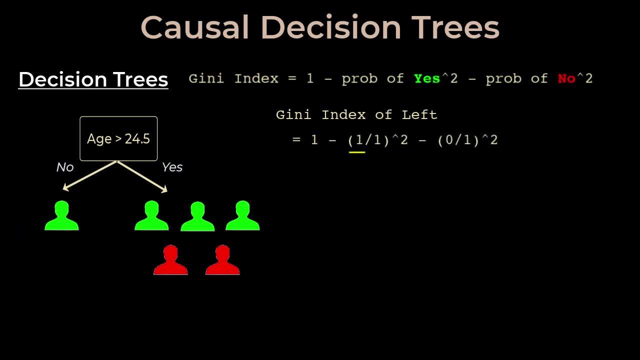 yes. this means that the probability of yes is one on one and the probability of no is zero, And substituting this in our Gini index equation, we get the Gini index of the left node as zero. Now for the right node, there were three yeses and two noes, so the probability of 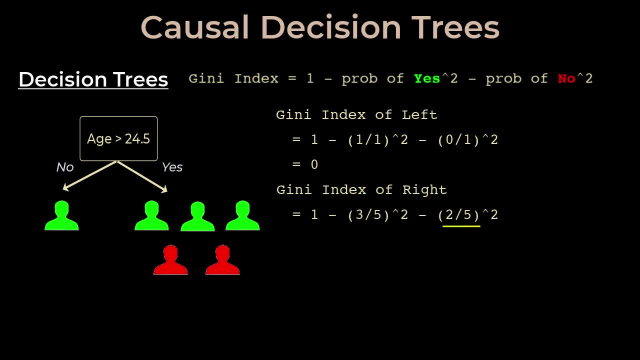 yes is three on five and the probability of no is two on five And using these values we get the Gini index of the right node as zero And the total Gini index is going to be the weighted average of these two values. Since only one out of the six samples went to the left node, its weight 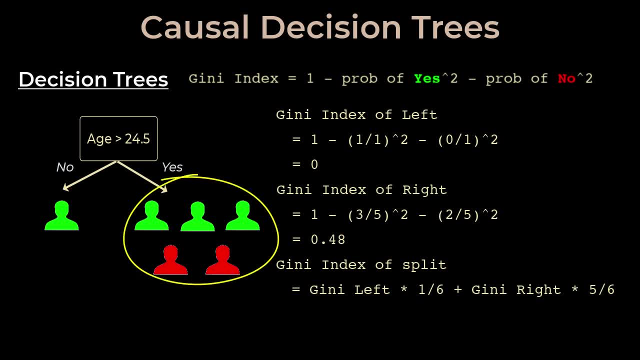 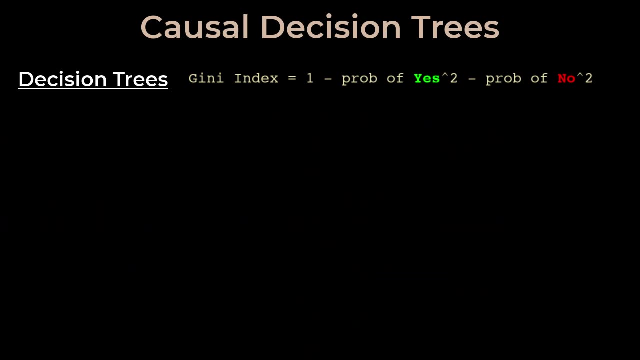 is one on six and the remaining five on six went to the right node, so its weight is five on six And substituting these values we get the final Gini index of the split as zero point four And like this we can compute the Gini index for all other age splits And I 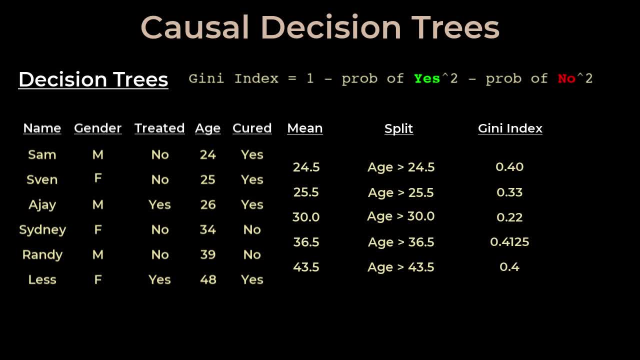 encourage you to walk through these numbers and do the math, just to make sure that you're on the same page here and you understand how these Gini indices are constructed. Now, in doing this math, we see that the age is greater than 30. split has the lowest Gini index here, Hence it is the best split. 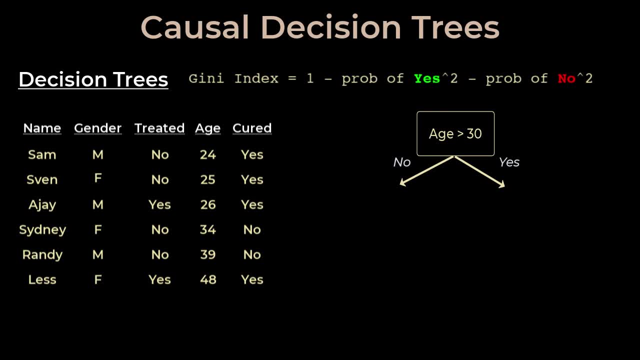 Let's see if we can compute the Gini index for all other age splits. Let's consider age greater than 30 split and pass our patients here just to see how the children look. We don't need to split the left child since it's Gini. 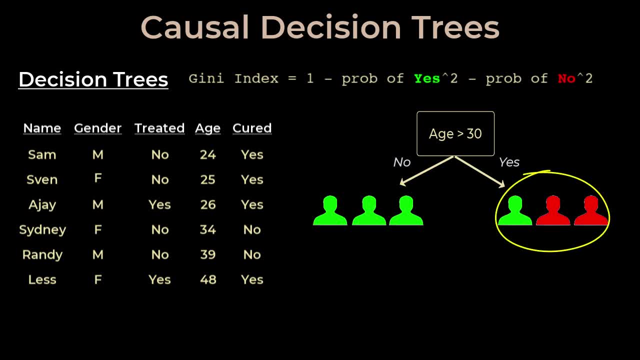 index is as low as it can go Now for the right child. we can check gender treatment and other age categories, as we did to further split this out. If we pass these three patients into the treatment node, the left node now has two. 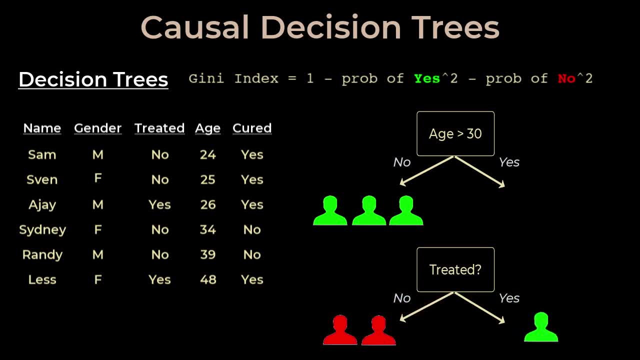 no's and the right node has a no. So now we know that the left node has two no's and the right node has a no. This is a perfect split, and the Gini index of this split will be zero. So you can stop here. We now assign a yes or no label to each leaf, depending on. 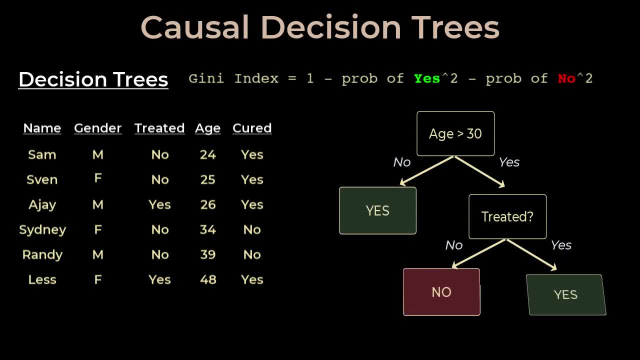 the majority And we're done. In this case we had pure nodes, but in practical situations we would see some impure nodes too. I hope the tree construction here is clear. The decision tree answers the question: determine if this person will be cured. 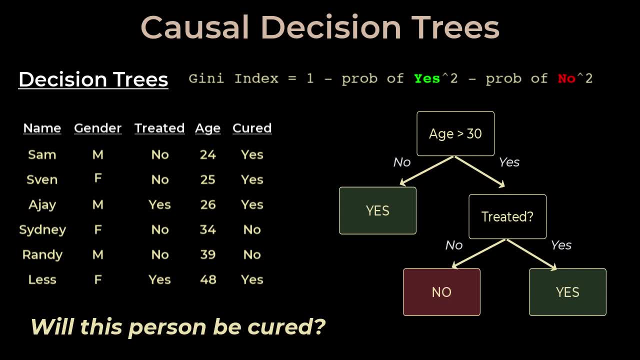 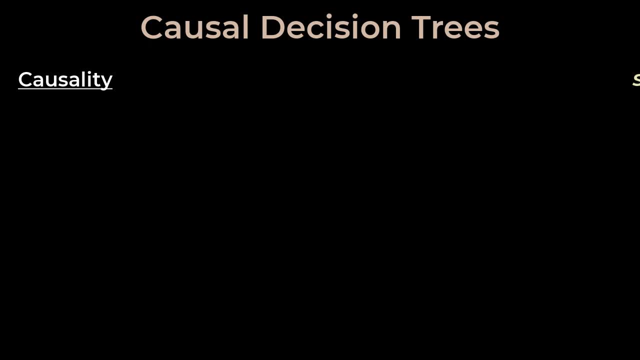 given a person's age, gender and whether they were given the treatment. But what if we want to go a step further and we want to answer the question? should we give this person the elixir? Answering this question means the tree. 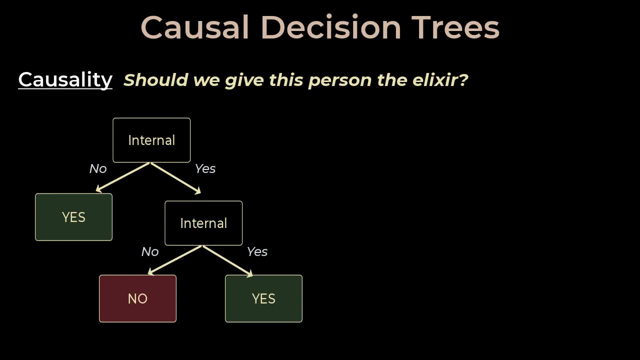 needs to understand if the treatment causes the flu to go away, and we can answer this by making a few modifications to the tree itself. The leaf nodes should be one of two outcomes: Yes, give this person the elixir. and no, don't give this person the elixir. And the internal nodes can be based off of one of 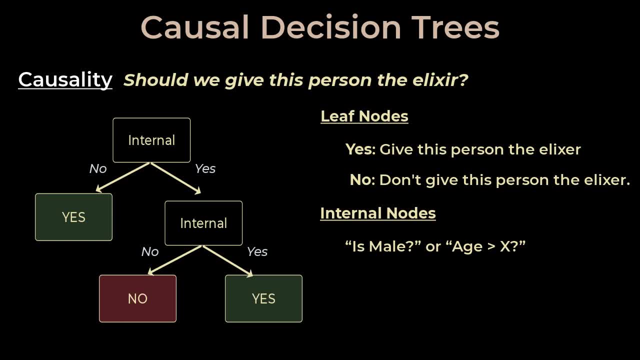 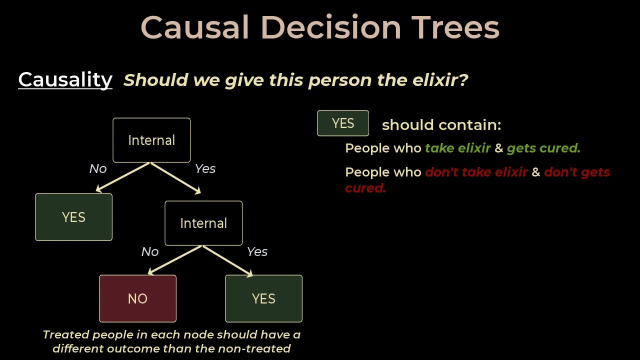 two variables now, gender and age, And the goal should be to choose internal nodes that can best split the yeses from the noes For the best split. those treated should behave as different as possible from those who are not treated. If a lot of treated people were cured in a node, then the non-treated people should not. 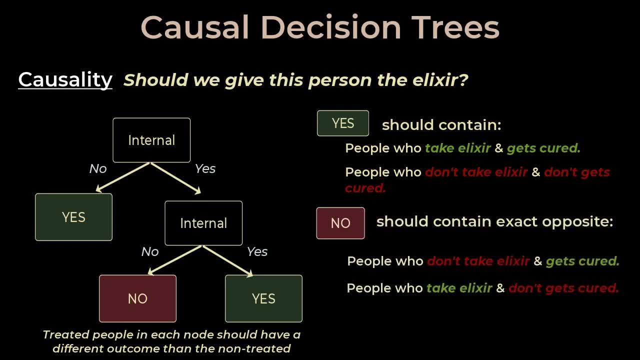 have been cured. This way, the node will be as pure as possible and we can assign a yes or a no to the node. And we quantify this node purity in this way with a metric called divergence. Larger the divergence, more pure is the node. 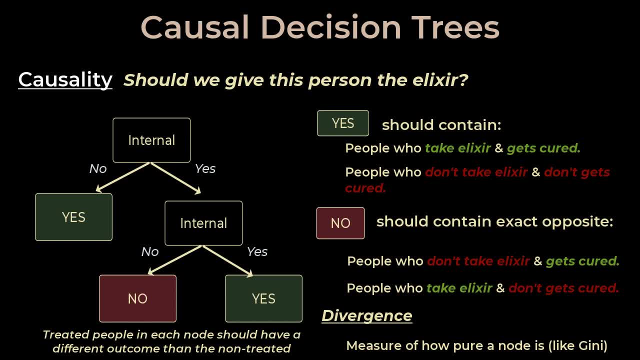 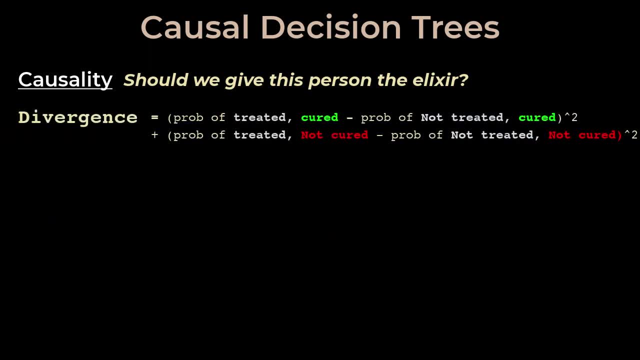 We want this divergence for a node to be as large as possible. So divergence will be the probability that a person is treated and cured, minus the probability that a person is not treated and is still cured. Square of that Plus the probability that a person is treated and not cured, minus the probability that. 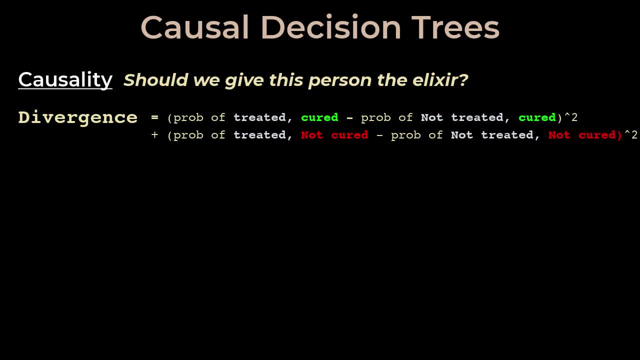 a person is not treated and doesn't get cured, And the square of this. Let's understand how well this metric works by constructing a new decision tree that answers the question: should we give this patient the treatment? So let's first consider gender as a potential split. 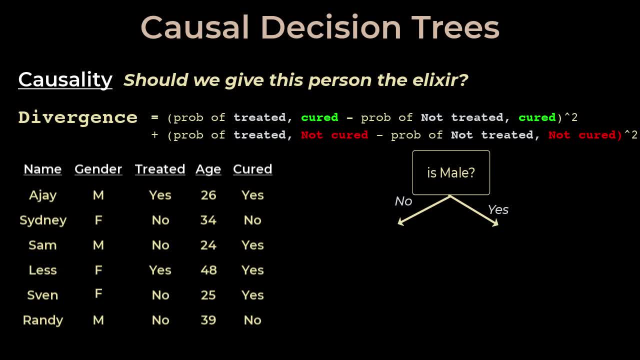 If we pass all of this, All the samples, through the decision node, then on the left node we get one treated person who got better, one non-treated person who got better and one non-treated person who did not get better, And on the right node we get the exact same thing. 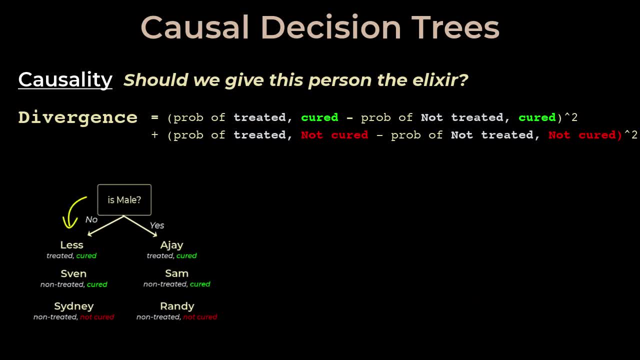 Let's calculate first the divergence of the left node, And we'll do this one term at a time. So the probability that a person is treated and cured Is the number of people who got cured divided by the number of people treated in that node. 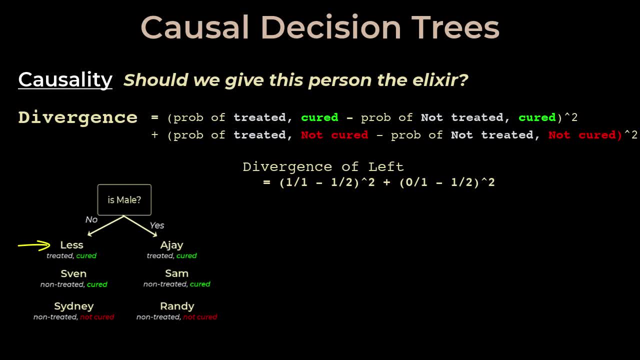 So we have one treated person who got better and the total number of treated people is just one, So it's one over one. The probability of not treated and cured is the number of people who were not treated and who got better, which is one. 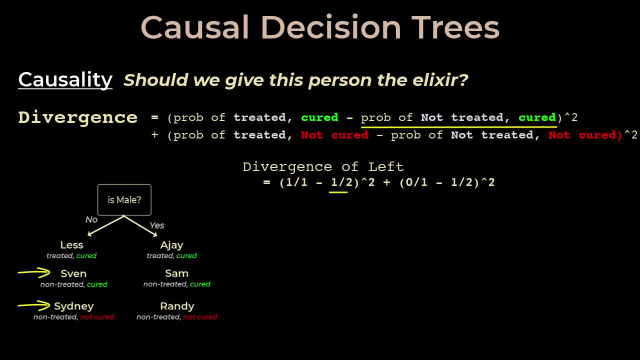 Divided by the total number of people who were not treated in that node, which is two. Okay, Okay. So the probability of a person being treated and not cured is the number of people who were treated and didn't get cured, which is zero. 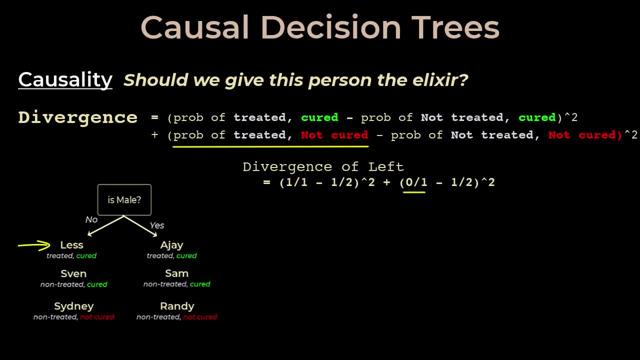 And so it's just zero over one, since one is the number of people who got treated And the final term is the probability that a person is not treated and not cured, which is one divided by the total number of people not treated in that node, which is two. 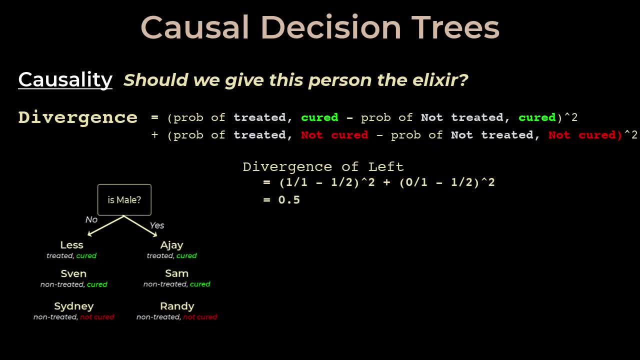 And so, plugging these values into the formulation, We get a divergence of the left node as 0.5.. Now, similarly, we also write out the divergence of the right node in the exact same way. And now, like we did before when we were doing the Gini index of the split, the divergence. 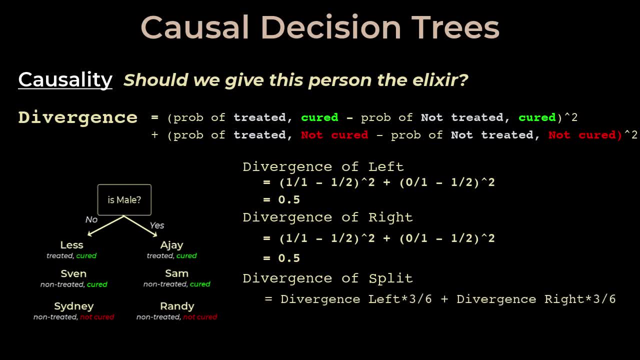 of this split will be the weighted average of the divergence of the left and right nodes. Okay, So the weight will be equivalent to depending on how many samples there were in that split. So in the left node we have three out of the total six participants. 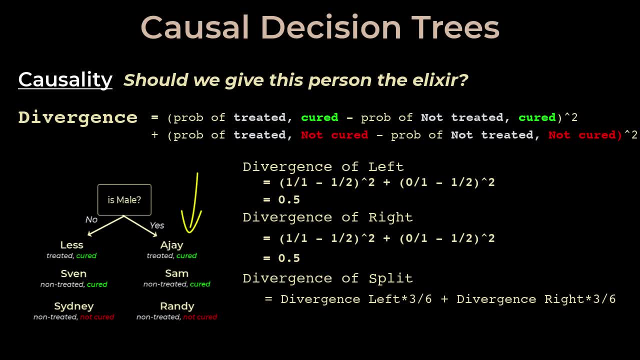 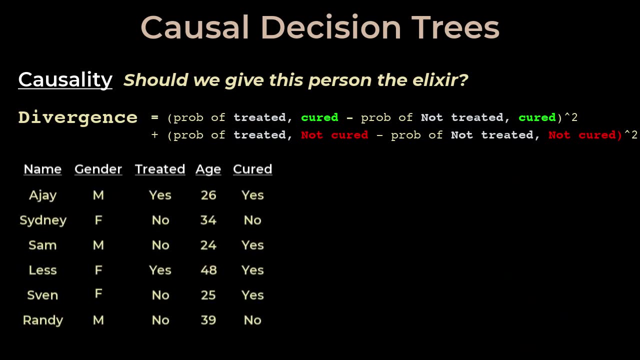 And in the right node we also had three on six of the total participants, And plugging these values in, we finally get a divergence of 0.5 for the split. Now let's consider age as a potential split And we'll use the thresholds that we determined before starting with. age is greater than 24.5.. 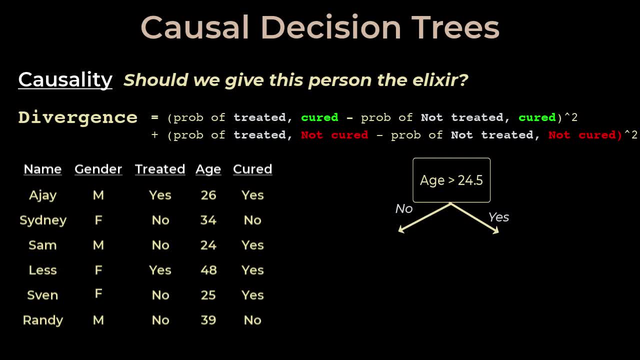 If we pass all the patients through this decision node, then on the left node we will end up with one non-treated person that got better And on the right node we will have two treated people who got better, one non-treated person who got better and two non-treated people who didn't get better. 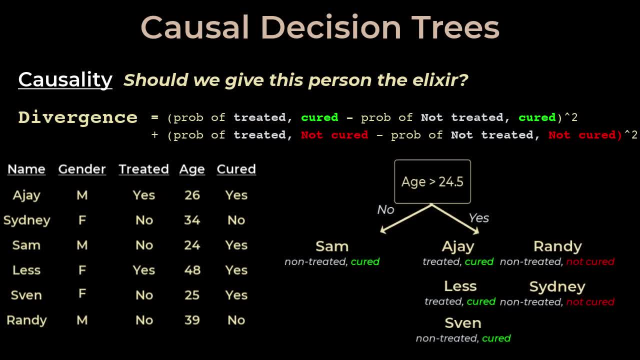 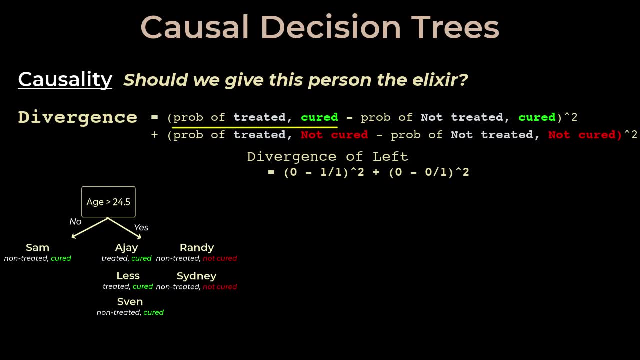 Okay, Now let's also again compute the divergence of the left node. So the first term: there are no people who got treated, So we'll leave it as 0 here. The next term is the number of non-treated people who got cured, which is going to be. 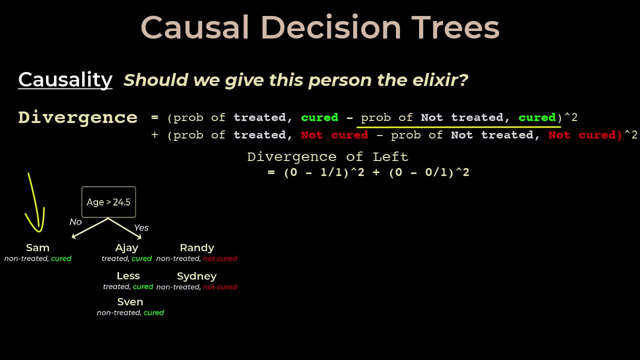 1, divided by the total number of non-treated people in that node, which is 1, hence 1 over 1.. Okay, Okay, Okay, 0, because there are no treated people, And the fourth term is going to be the number of non-treated people who didn't get better. 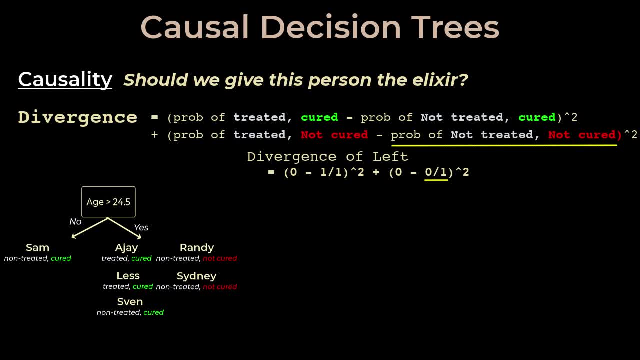 which is 0,, divided by the total number of non-treated people, which is 1.. And plugging these values in, we get a divergence of the left node as 1.. Now for the right node. we have a lot more participants here. 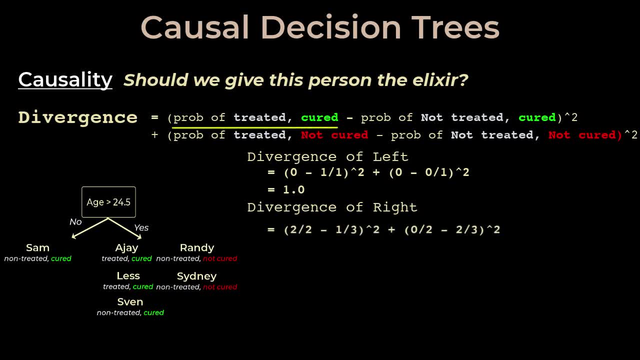 The first term is the number of treated people, So the number of non-treated people who got cured, which is 2, divided by the total number of people who were treated, which is also 2.. Hence 2 over 2.. The second term is the number of non-treated people who got cured, which is 1, divided. 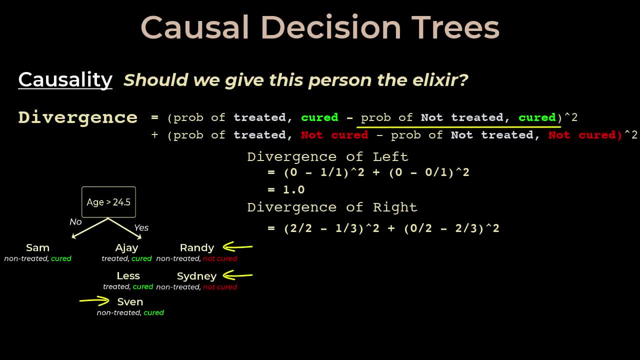 by the total number of non-treated people, which is 3.. Now the third term is the number of treated people who didn't get cured, which is 0.. Okay, Okay, 0, divided by the total number of treated people, which is 2.. 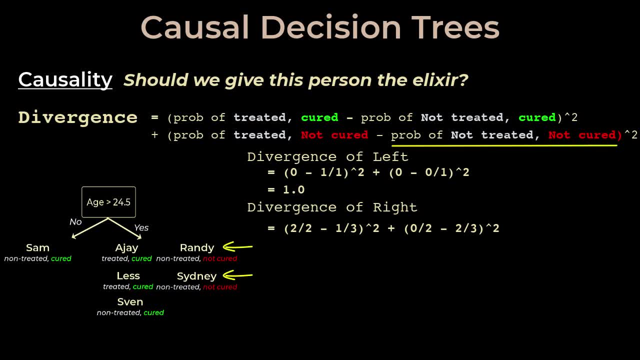 And then we have the total number of non-treated people who didn't get cured, which is 2, divided by the total number of non-treated people, that is 3.. And substituting these values, we get the divergence of the right node as 0.888.. 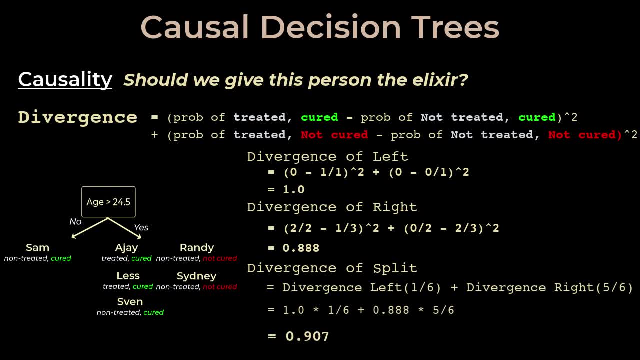 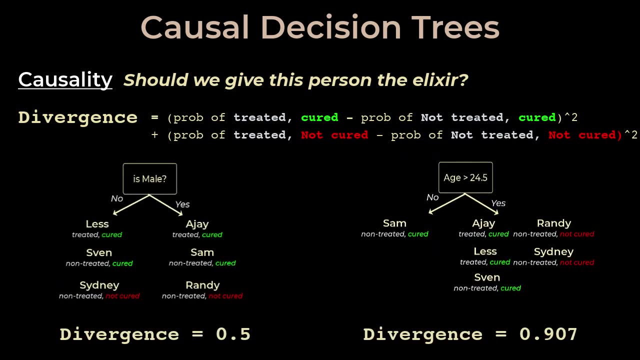 And then computing the weighted average of the left and the right nodes, we get 0.907 as the divergence of the age greater than 24.5 split. So it looks like the divergence of this age split is higher than that of the gender split. 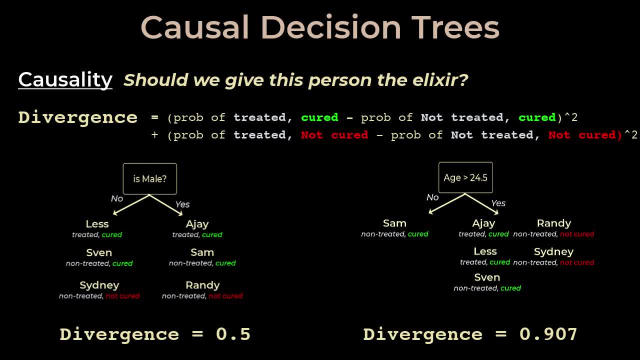 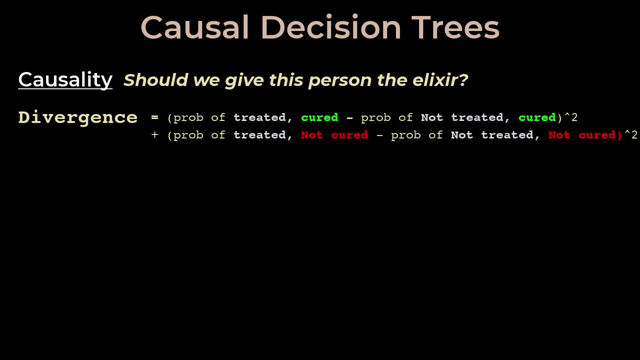 And this means that the split of age leads to more pure nodes and is indicative of a better split. And like this, we have the divergence of the age greater than 24.5.. So it looks like the divergence of this age split is higher than that of the gender split. 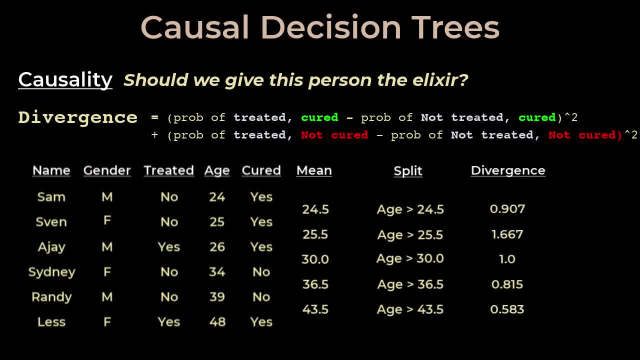 And like this we have the divergence of the age greater than 24.5.. And like this we have the divergence of the age greater than 24.5.. So we can compute the divergence for each age split. We notice the highest divergence in the case of age greater than 25.5.. 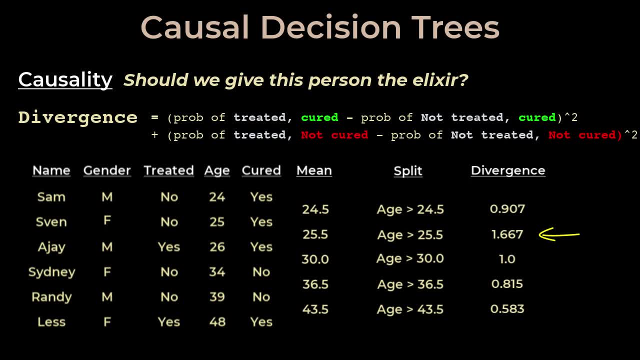 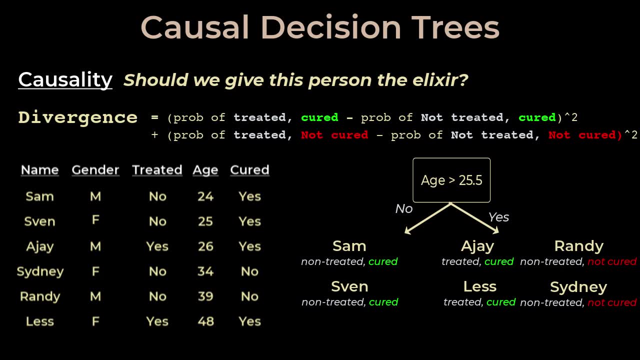 And so we make use of this as the split. Looking at the result of this split in the right node, all the treated people got better and the untreated people didn't get better. This is a very pure node where we tell everyone: yes, take the elixir. This is reflected in the divergence that is also.